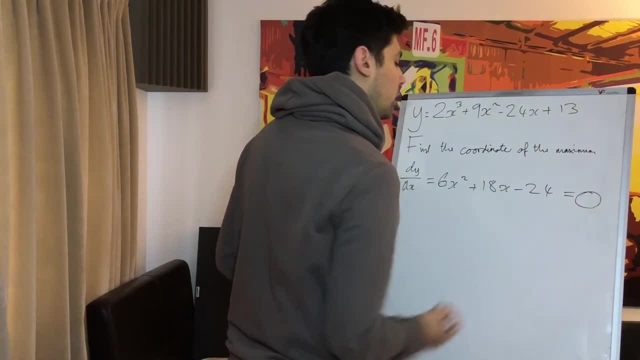 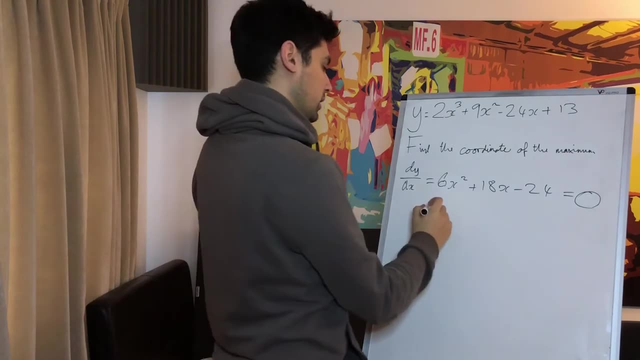 needs to equal zero. So the first thing I notice here is that all of these individuals are divisible by six. So let's fucking get rid of that. Let's do it. Divide everything by six, We've got x squared plus 3x minus 4.. Much nicer looking now, So 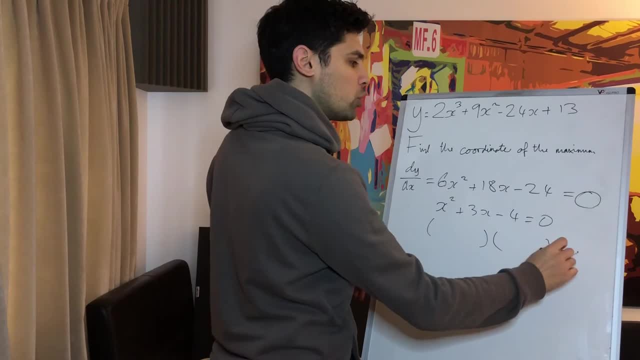 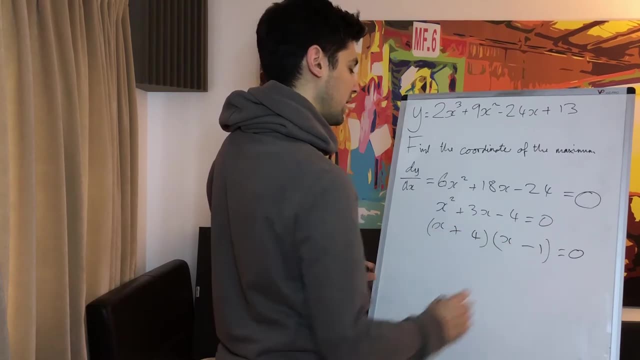 let's factorise this. Whenever we see a quadratic, our first thought should be: should we be factorising this? x, x, 4, 1, positive, 4, negative 1.. That means x is minus 4 and x. 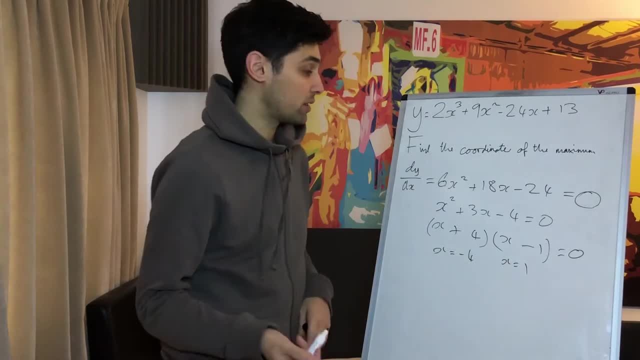 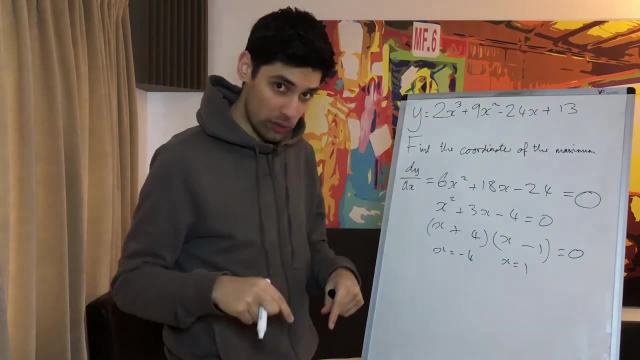 is 1.. These are the x coordinates of the turning points. Now, one's going to be a maximum, one's going to be a minimum. How do we know which one's which? Well, we need to find the second derivative. So that's going to be d2y over dx squared. 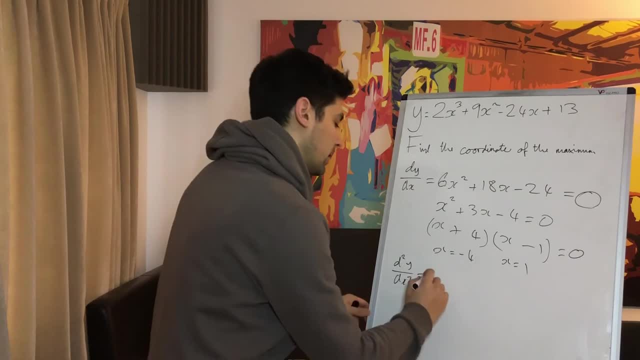 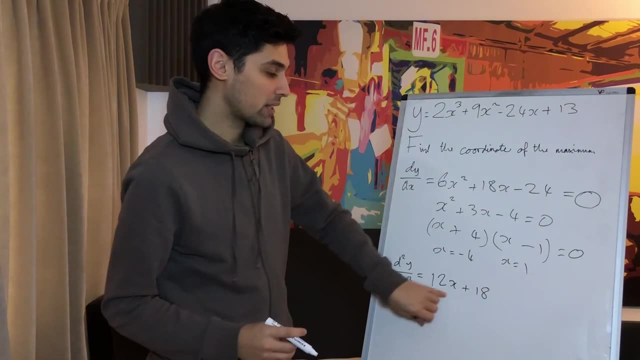 And we just differentiate this again. So we're going to bring the 2 down in front to make it 12x plus 18.. Then we're just going to plug in the minus 4 for x and the 1 for x. Now 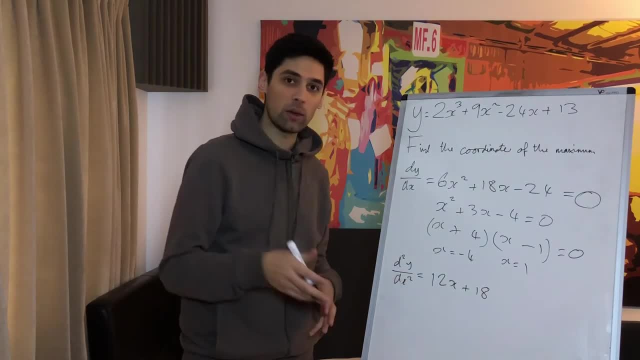 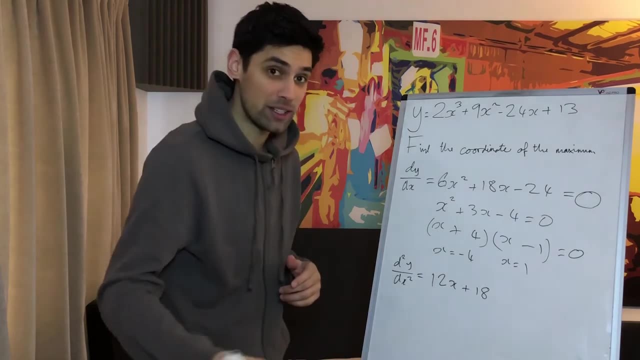 it's a little bit counterintuitive here, because the way we decide which one is a minimum and which one is a maximum is based on whether this answer is positive or negative. So we're going to say it's a minimum. And the reason I say it's counterintuitive is because if 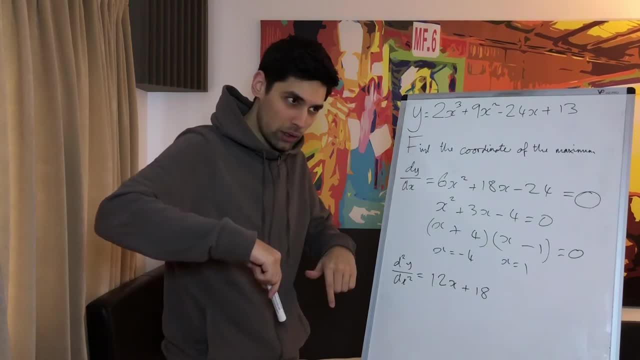 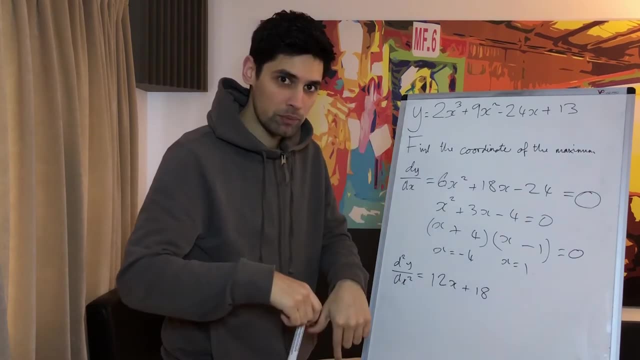 the double differential. the double derivative is negative, then that point is a maximum, And if the double derivative is positive, then it's a minimum. So we've got to be really careful about that. Just remember it's that way around. Now, just to save a little bit, 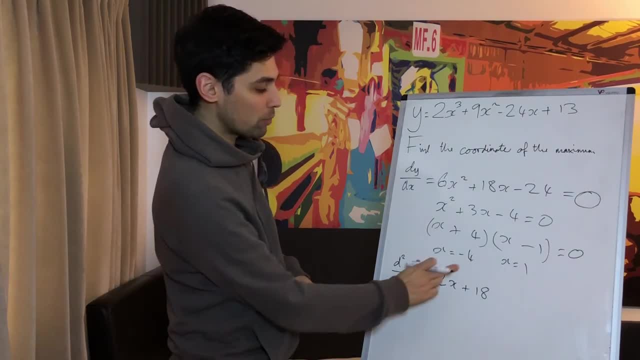 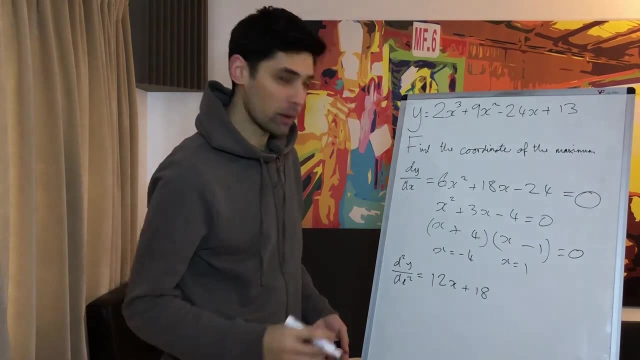 of time and I'm running out of space. we can clearly see that if we plug in the minus 4 into there, that's going to create minus 48. plus 18 is minus 30. So that one is going to be a maximum- Sorry, maximum, because we get a negative. See, even I fucking get. 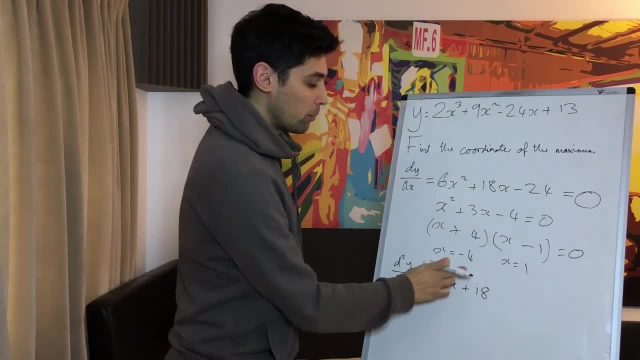 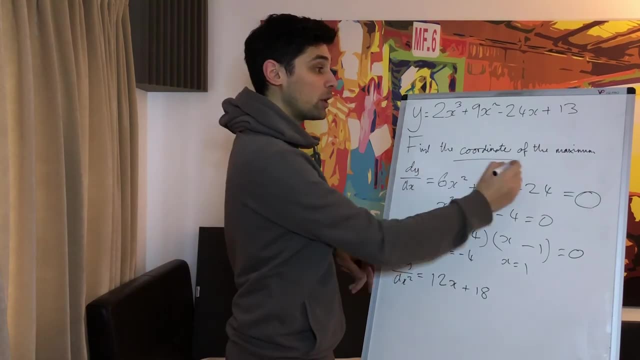 it wrong sometimes Just need to always be switched on. So the minus 4 gives us a negative value, which means the minus 4 is the coordinate of the maximum. The question is asking for the coordinates, not just the x-coordinate. So we know the x-coordinate is minus 4.. To